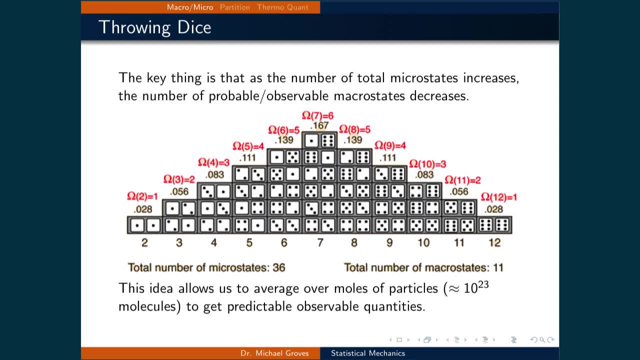 possible face value combinations of two dice, ranged according to their total. A micro state in this case is the face value of the two dice. So a micro state would be when one dice reads one and the other also reads one, Since we can distinguish the two dice, then a face value of five and two. 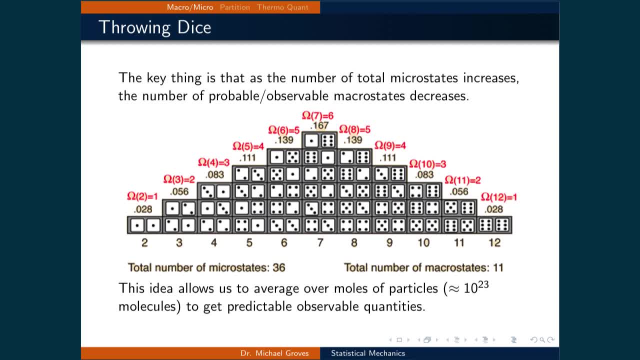 is different from two and five and are counted as two different micro states. The macro state in this example is the total from both dice. Since each micro state is equally likely, then the number of micro states in a macro state determines how likely a given macro state is, As can be seen in the image. 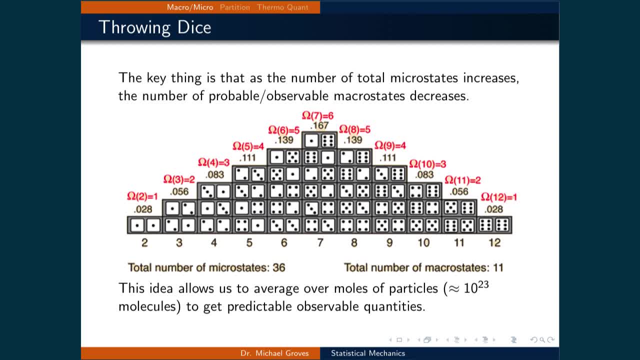 seven is the most probable macro state, since there are six combinations of micro states that give seven. Two and twelve are the least likely macro states, since there is only one micro state for each. There are a total of 36 micro states and 11 macro states for this system. An important observation is: 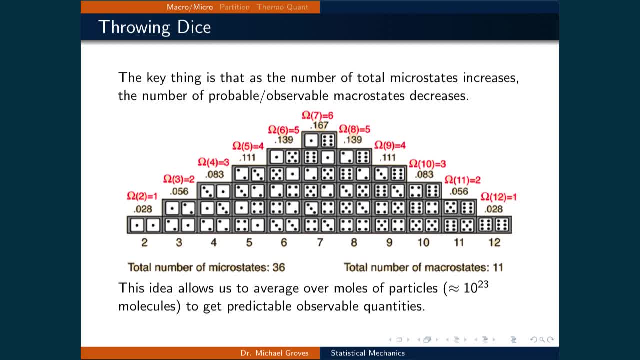 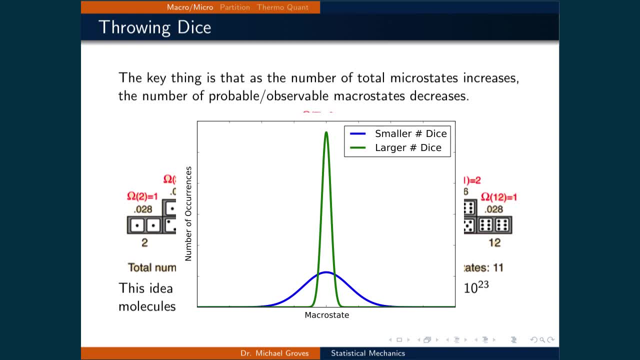 that as the number of total micro states increases, the number of probable or observable macro states decreases. In the dice example, increasing the number of micro states means throwing more dice. If we were to throw more dice, say 10 or 100, the broad distribution seen with the two dice becomes: 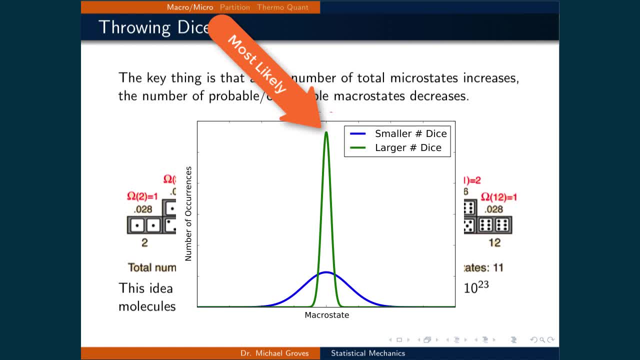 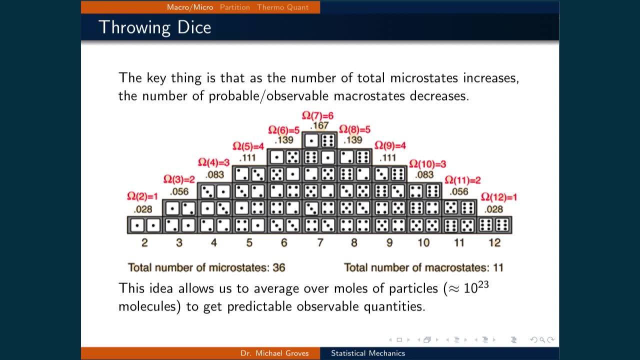 much thinner, The most likely macro state becomes very probable relative to all others. This phenomenon is what allows us to average over moles of particles and get predictable, observable quantities, since they tend to be the most probable. If we were to throw more dice, then the number of 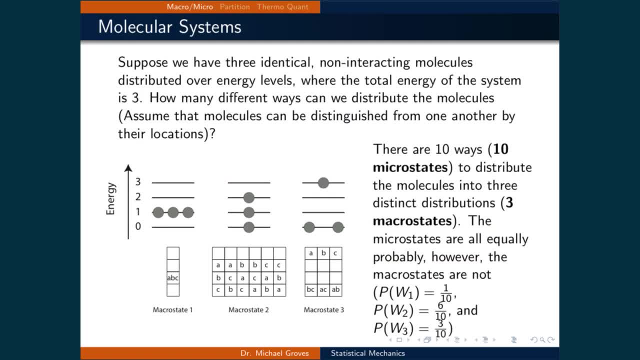 micro states would be the only probable ones. Consider a second example. Suppose we have three identical non-interacting molecules distributed over energy levels where the total energy of the system is equal to three. How many different ways can we distribute the molecules? Assume that. 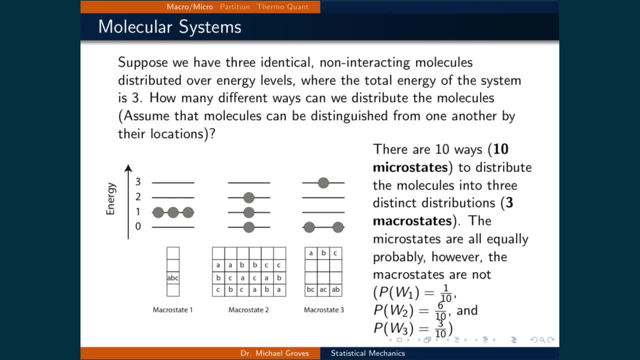 the molecules can be distinguished from one another by their locations. The illustration on the left shows that there are in general three ways to distribute the molecules in the energy levels. These are the macro states. For each macro state there are different number of microstates. For macrostate 1, there is: 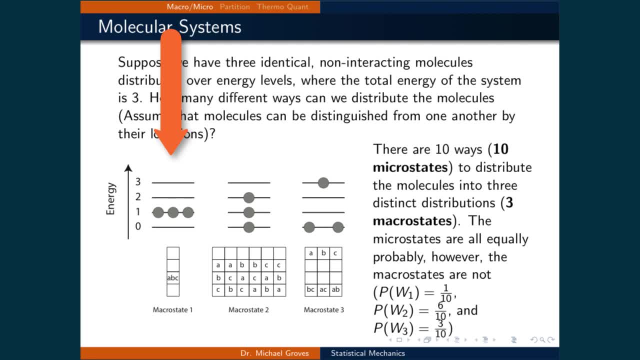 only one way to put all three molecules into energy level 1.. For macrostate 2, there are six ways to arrange the three molecules on their own in energy levels 0,, 1, and 2.. Finally, there are three ways to distribute the three molecules where. 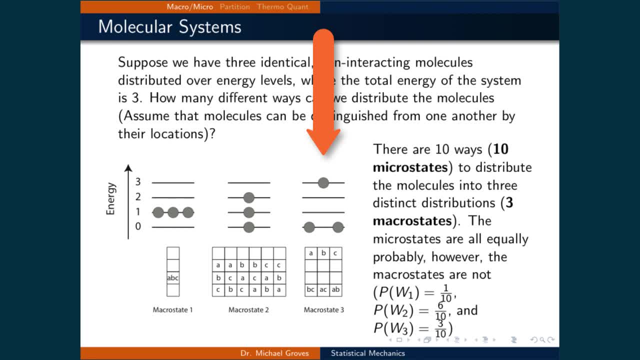 one is an energy level 3 and the other two are in energy level 0.. Since there are ten ways to arrange the molecules so that the total energy is 3,, then that means the most probable macrostate is number 2.. The general formula for 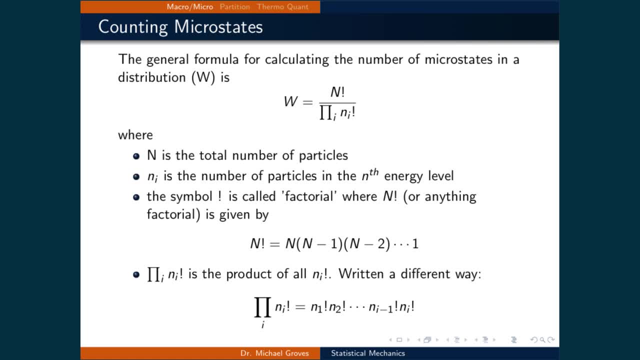 calculating the number of microstates in a distribution. W is equal to n factorial divided by the product of ni factorial. and this is where n is the total number of particles, ni is the number of particles in the nth energy level. the exclamation mark is called factorial where n factorial or anything factorial. 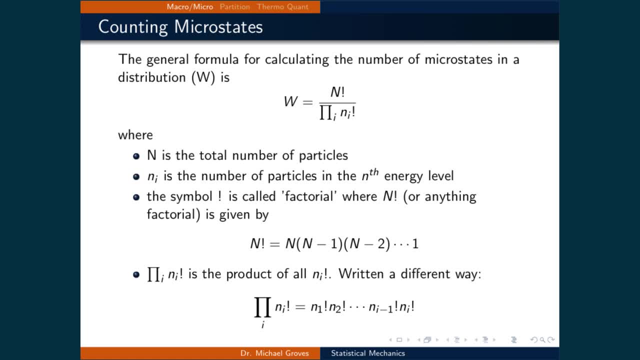 is given by n times n minus n. n is equal to n minus 1 times n minus 2, all the way down until it's times 1.. As a side note, 0 factorial is also equal to 1.. The large pie symbol means the product. 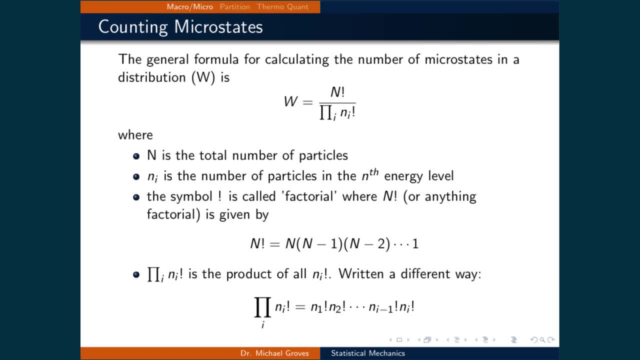 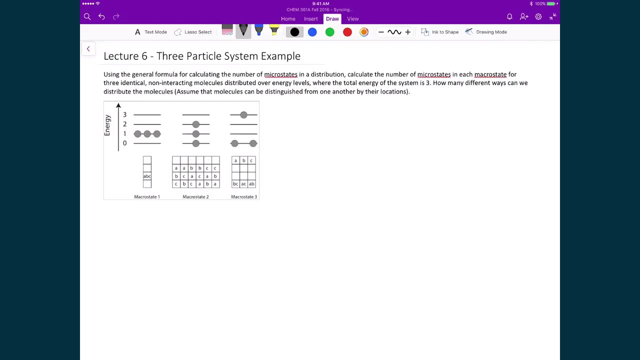 of all that follows. In this case it is referring to the product of all ni factorial. In a different way, it would be written as n1- factorial times, n2 factorial, all the way to ni minus 1 factorial, ni factorial. Let's use this: 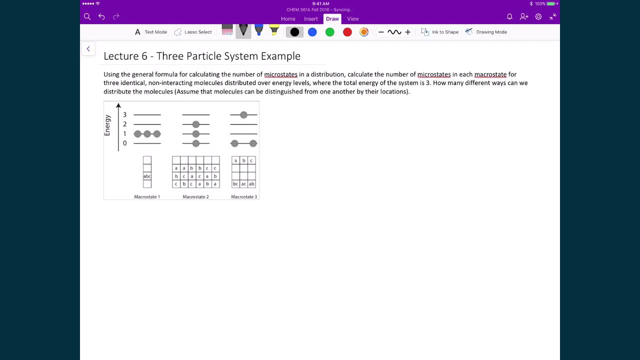 now, in practice, to determine the number of microstates in a distribution, using the exact same problem that we had already analyzed with our three particle system, where what we're trying to do is just have three identical non-interacting molecules distributed over energy levels where the total energy is equal to 3.. 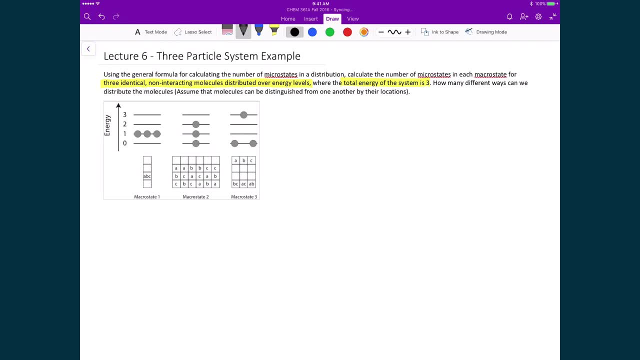 And so what we're trying to do is again just determine how many microstates exist in each of the three macrostates, And so the way that we calculate this, as was shown on the previous slide, was that we would then take n factorial divided by the product, over i of ni factorial. And so in this case, since we've 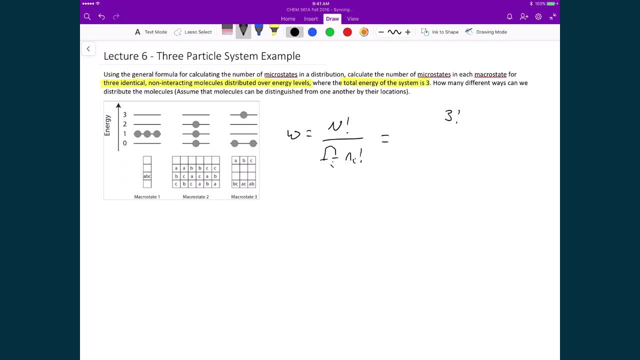 got three particles in our system. that means on top we're going to have 3 factorial, And on the bottom, well, this pi, this capital pi sign, just means the product of what follows, And i basically is going to be equal to 0,, 1,, 2, and 3.. 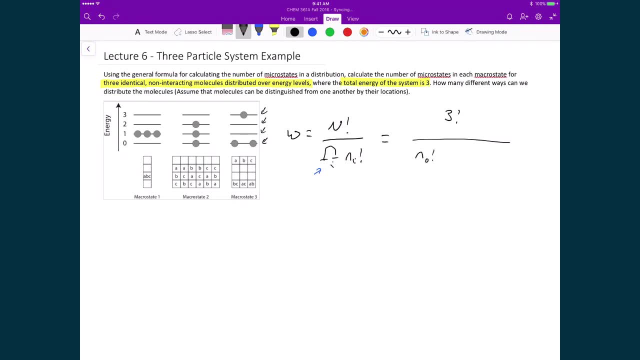 So that means, on the bottom, what we're going to have is the number of particles in the system, The zeroth energy level factorial times, the number in the first energy level factorial times, the number in the second energy level factorial times, the number in the third energy level factorial, And so we're going to use this general 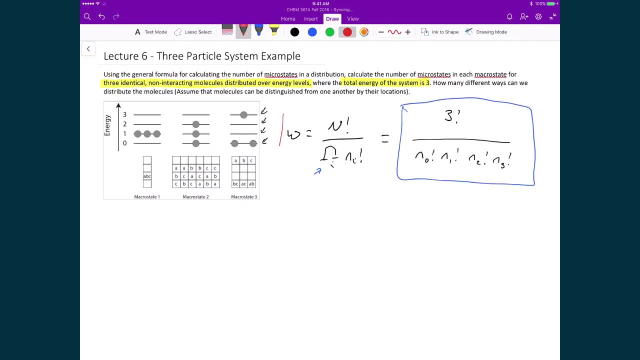 expression, then, based on the original definition, to determine how many microstates exist in each of the three macrostates that we examined previously. Let's now apply this to each of the macrostates. So for macrostate number one we have, starting with the general definition, we have n factorial divided. 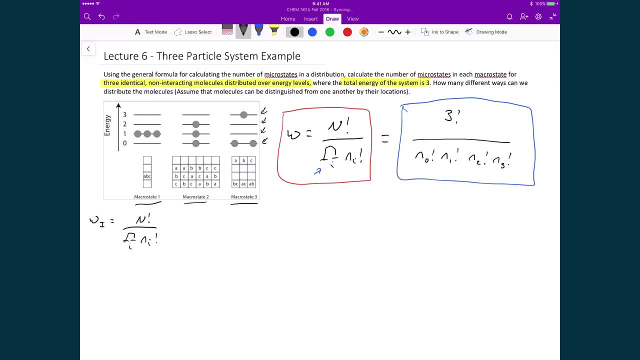 by the product over i of ni factorial. For this system, and like for the other three, we've got three factorial on top And on the bottom we're basically again taking the product of the number of particles sitting in each of the energy levels. So n0, there are zero particles in it. n1, there are three. 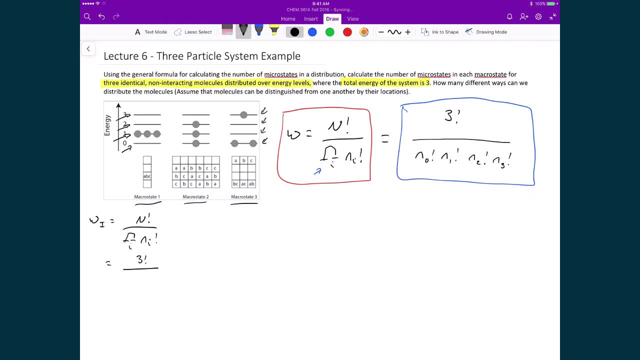 n2, there are zero And n3, there are zero. So that means I'm going to write 0 factorial, 3 factorial, 0 factorial, 0 factorial. Now we know that each of these 0 factorials, they're just equal to 1, and so what? 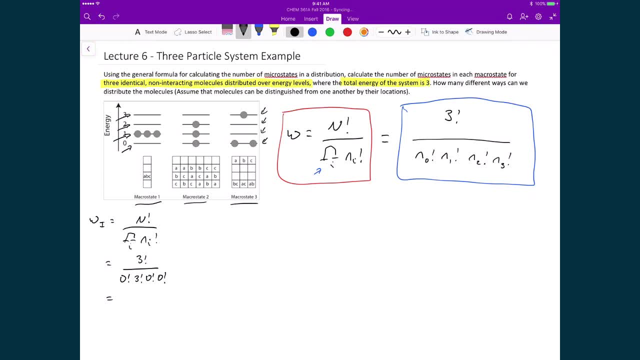 we're left with is 3 factorial divided by 3 factorial, which means that there is only one microstate in macrostate 1, which is an answer that we already showed to ourselves and we can see in the image Moving on to macrostate number. 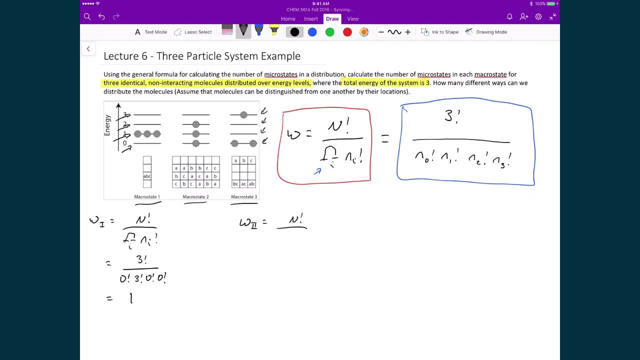 2, we again, we can start with the general definition: n factorial with a product over i of ni factorial. Well, in this case we still have 3 factorial. on top, the number of molecules haven't changed. On the bottom, well, we have one. 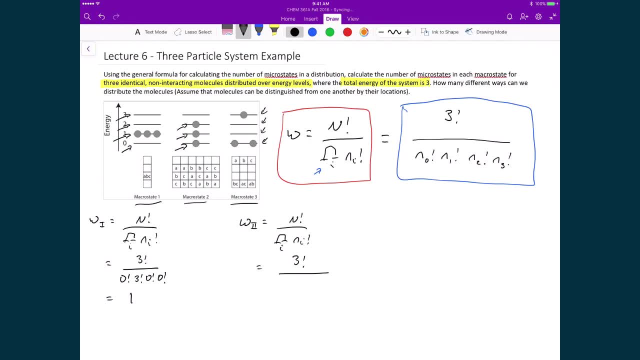 particle in n0,, one particle in n1, one particle in n2, and zero particles in n3. So that means we have 1 factorial times 1 factorial times 1 factorial times 0. And that this denominator is 1 times 1 times 1 times 1, so it's just 1.. 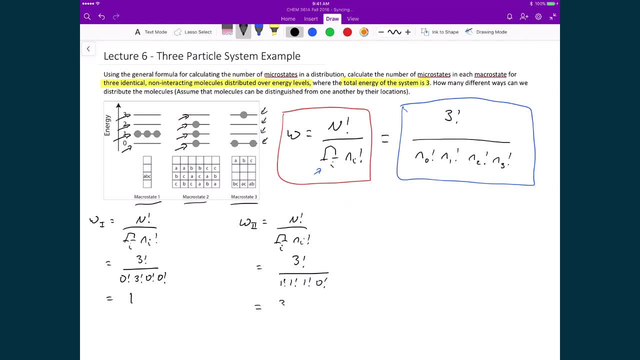 That means we're left with 3 factorial on top, 3 times 2 times 1 over 1, which means that we have a total of 6 microstates in macrostate 2.. Let's now determine the number of microstates in macrostate number 3.. Here again n. 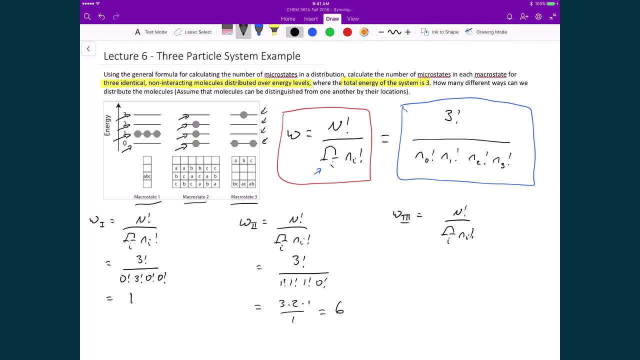 factorial divided by the product over i of ni factorial, What that gives me again 3 factorial on top. Well, here we have 2 in n0,, 0 in n1,, 0 in n2, and 1 in n3.. So we have 2 factorial times, 0 factorial times 0. 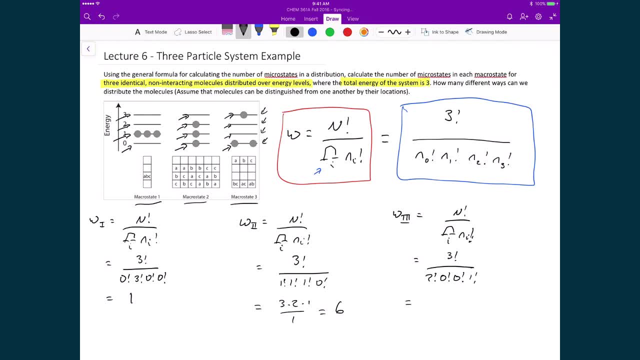 factorial times 1 factorial, And so in this case, again the zeros and the 1 factorials, they're just equal to 1.. And so what we're left with is 3 times 2 times 1, divided by 2 times 1.. And so in the end what we have is 3. 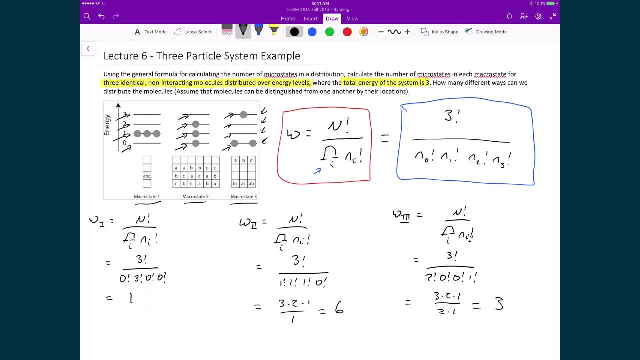 microstates in macrostate number 3.. Now, one point I'd like to stress again is this fact that each microstate is equally probable of occurring, And so that means that we have, over the sum of all of these different microstates, we have 10 in total, And so if each of these then are equally likely, then the one or 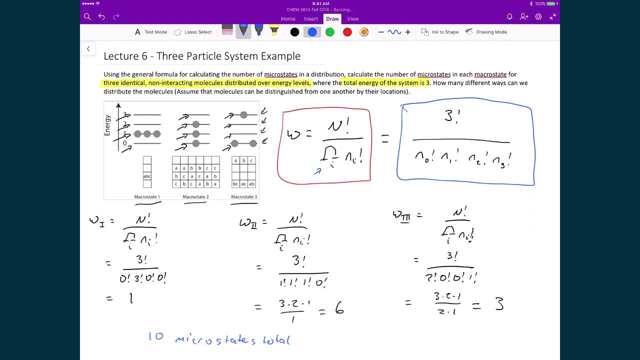 the macrostate that has the most number of microstates is going to be the one that we're going to observe the most. It's the one that's most likely, And so that means, then, that in this case, given this specific system, macrostate number 2 is going to be the one that we're going to see the most, or 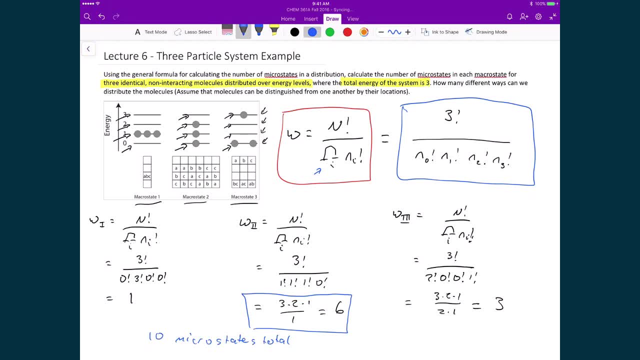 that we're going to measure the most, because it has 6 microstates, Or in other words, it has the most microstates out of all three. And then, in this case, micro or macrostate, number 1 is the one we will least see, since there's only one. 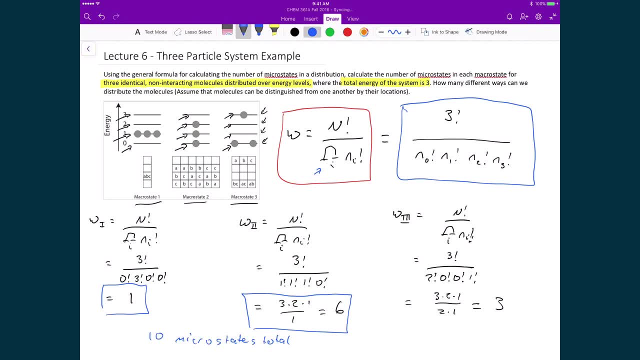 microstate that makes up this one state. What this says to us also is that if we are in macrostate number 1,, if we somehow found ourselves in that state, we would tend to then move towards macrostate number 2,, since it is more likely that we 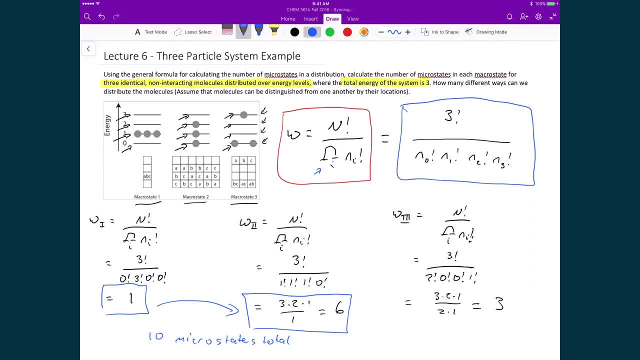 will find it, Or there's six possibilities out of ten as opposed to one possibly out of ten. That is, if the system matures or changes into something else, that it would then tend to change into macrostate number 2.. Similarly, if we found 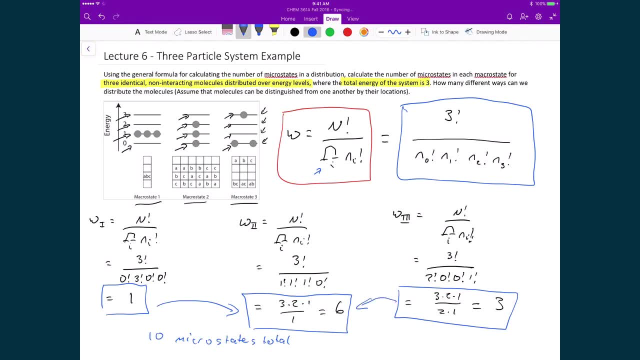 ourselves in macrostate number 3, again, we would tend to move towards macrostate number 2 when the system changes, simply because it is just more likely that we're going to find ourselves in macrostate number 2.. It's just more likely that we would end up in macrostate number 2, because there's